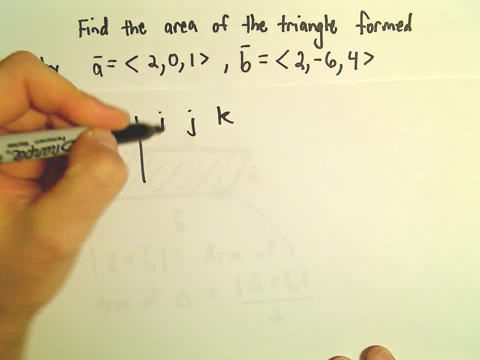 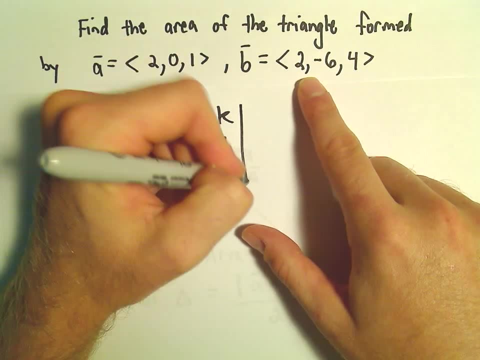 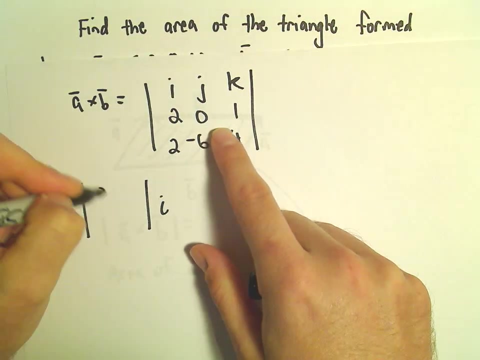 we've got I, J, K. Vector A has components 2,, 0,, 1.. Vector B has components 2, negative 6, 4.. Alright, so if you imagine covering up the I column, we'll be left with 0, 1, negative 6, and 4.. 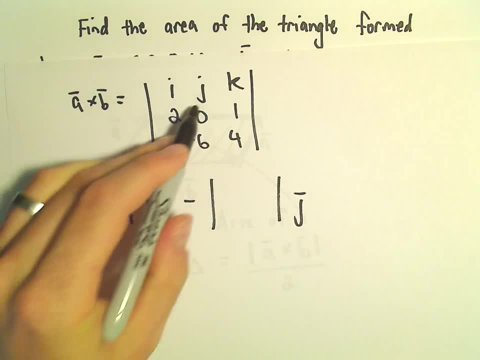 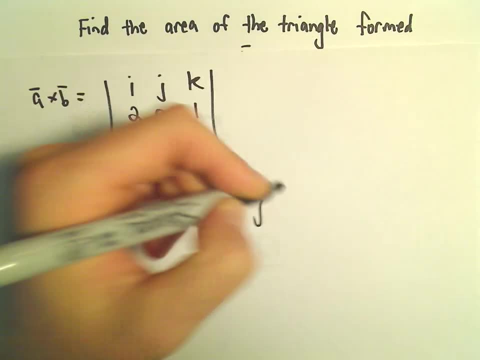 We'll subtract away the J component, So J. if we cover up that column, we're left with 2, 1, 2, 4.. So 2, 1, 2, 4.. And then we'll add to that our K component. 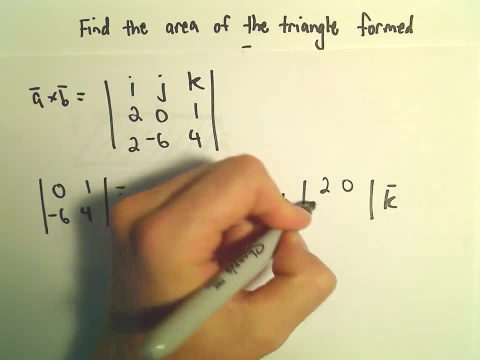 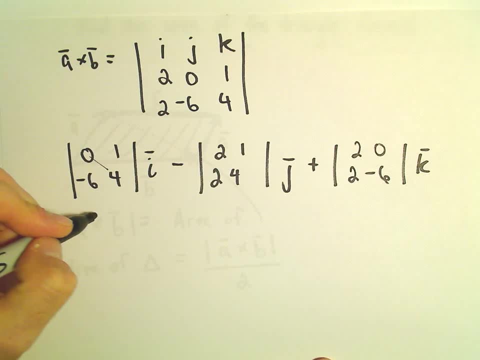 So then we'll be left with 2, 0,, 2, negative 6.. So let's see: 0 minus 4 is 0. We'll get minus negative 6.. So that'll leave us with positive 6I. 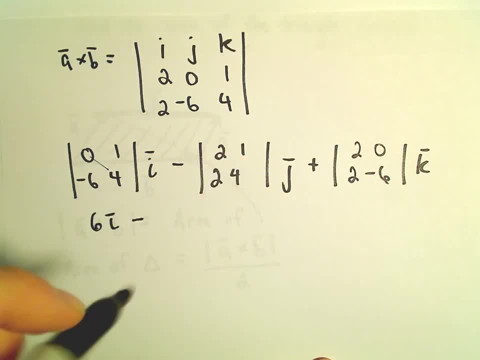 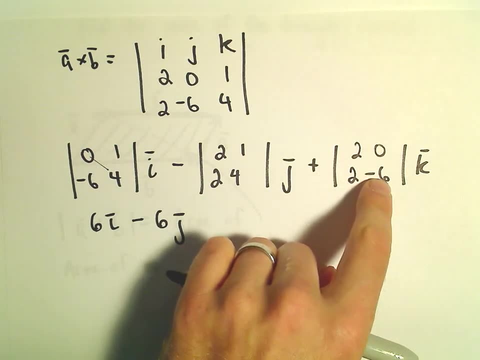 Minus, we'll have 2 times 4, which is 8 minus 2.. So that'll leave us with a negative 6J, And then it looks like we have negative 12 minus 0.. So let's see: negative 12 minus 0. 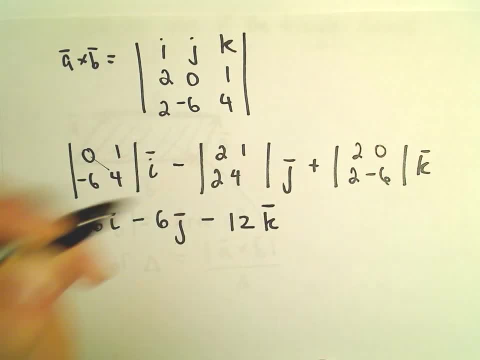 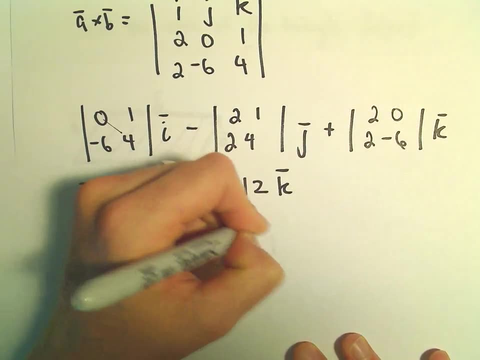 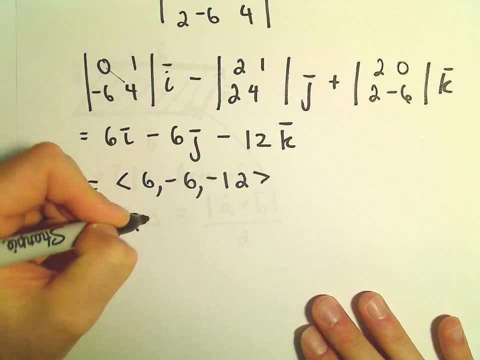 is just going to leave us with well negative 12 times K. So it says the cross product has components 6, negative 6, negative 12.. And now we'll just find the magnitude of this. So that says the magnitude of A cross B. 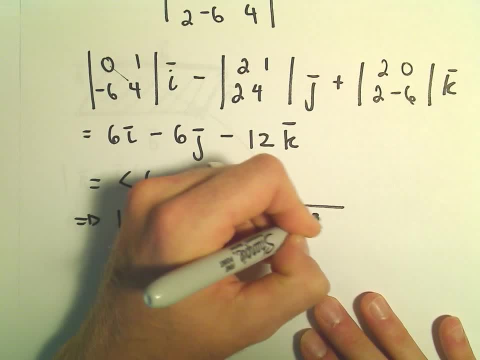 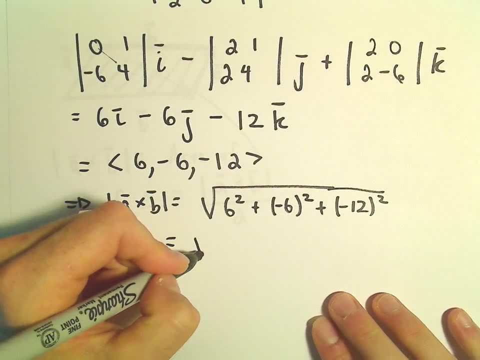 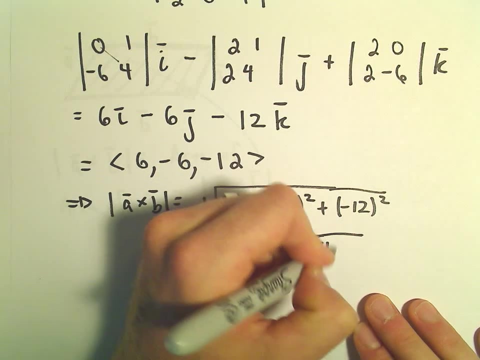 well, that's going to be 6 squared plus negative 6 squared plus negative 12 squared. Well, let's see: 6 squared is 36.. Negative 6 squared is also 36.. Negative 12 squared will be 144.. 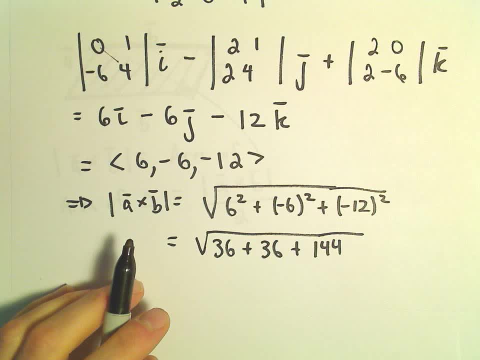 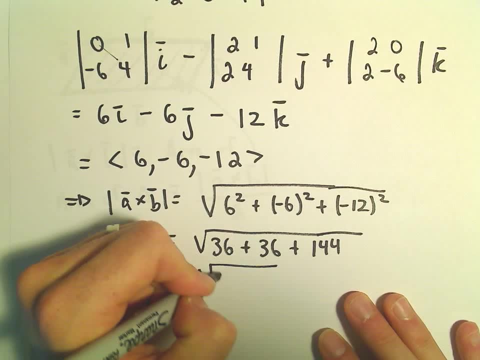 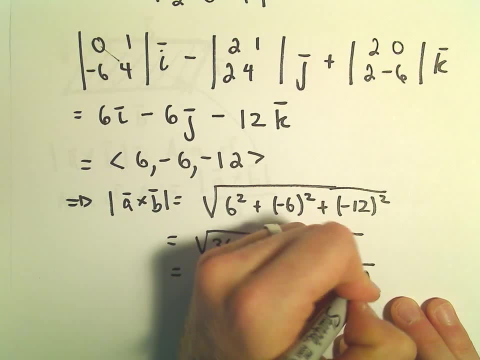 So let's see if we simplify that: 144,, I guess, plus 72.. That's going to leave us with let's see. so I guess that'll leave us with a square root of what. How about 216??